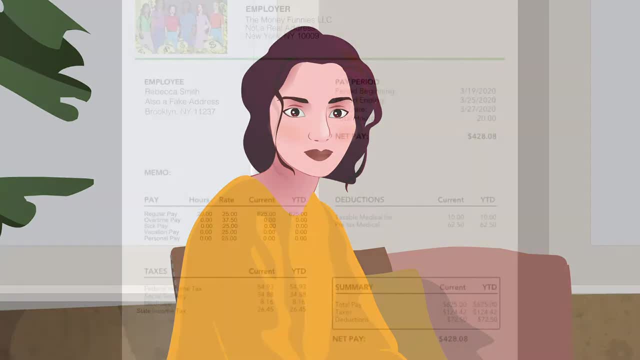 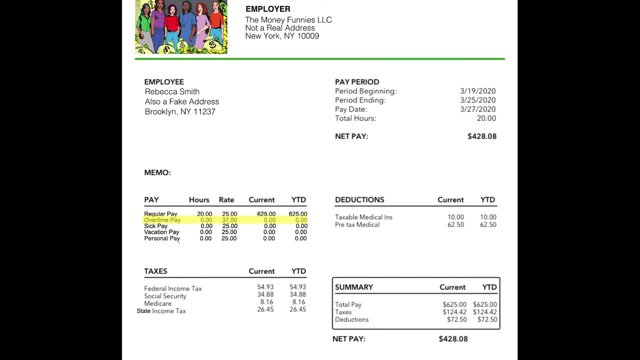 So when we were 16, paychecks looked a bit different. This is a more modern pay stub. from my direct deposit You can see the different hours. I worked Regular overtime. I didn't get paid time off, but there's a space for it here on the paycheck stub. 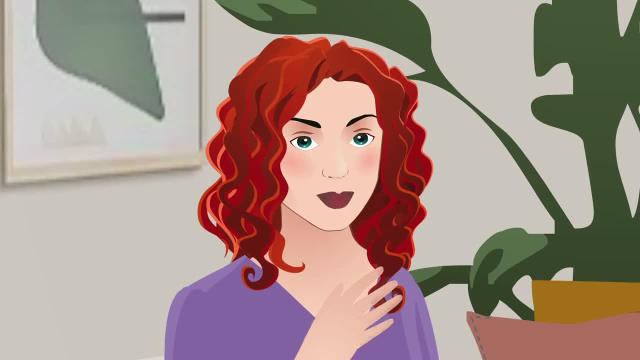 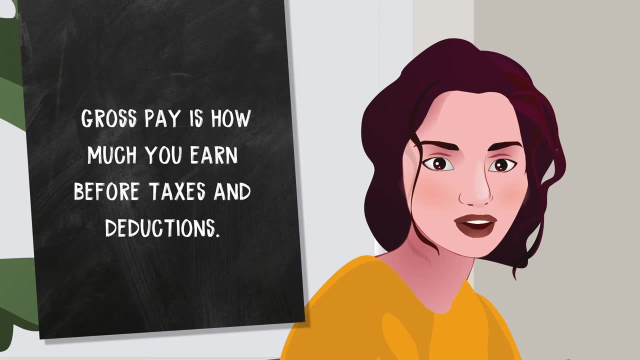 Vacation, sick, personal. So that's how much you earned in the paycheck. That was my gross pay, yes, In other words, the amount I earned before taxes and deductions. It's the amount often listed on a job posting as the amount made. 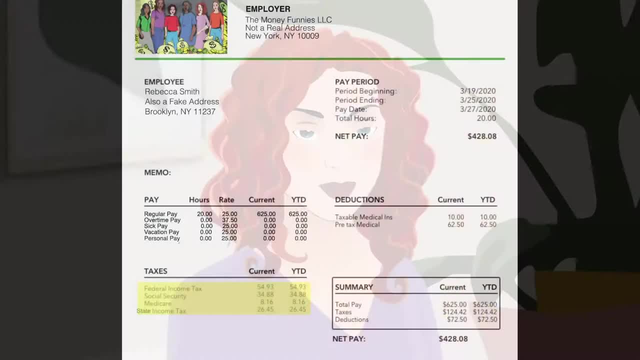 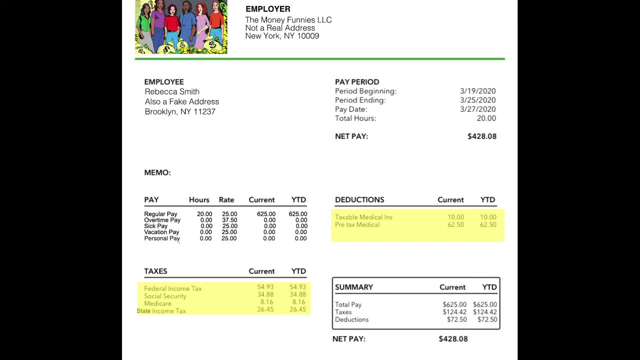 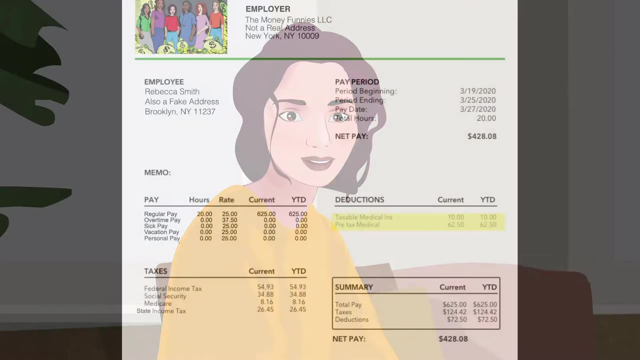 Say $12 per hour or $40,000 a year, Got it? You can see a variety of both taxes and deductions. The non-tax deductions are going to vary depending on your job and benefits. What do you mean? Well, you can see here that some money has been deducted from my gross pay to go toward my health insurance. 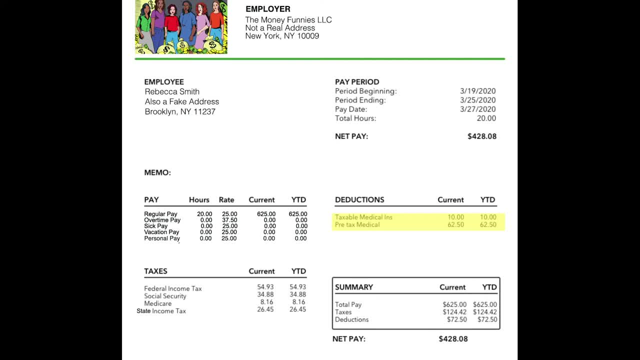 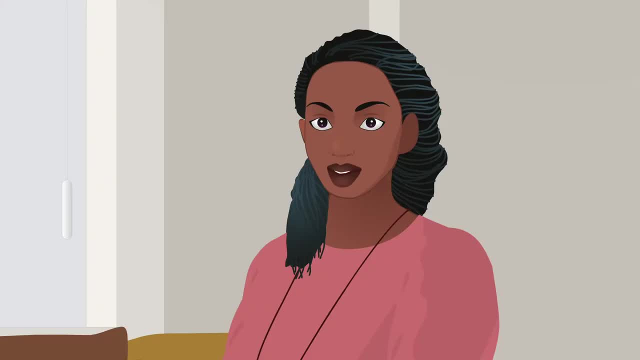 I get insurance through my employer, like many Americans, but have to pay a portion of the premium. That amount is deducted directly from my paycheck. So if we don't get health care through our job, it won't be on there, Right? Either it won't be there at all or the line will say $0.. Make sense. Yes, On to the taxes, The specific amount deducted will vary based on your income, But the types of taxes and the percentage of your income they cost are more based on where you live and work. Going down this list, we have federal income tax. 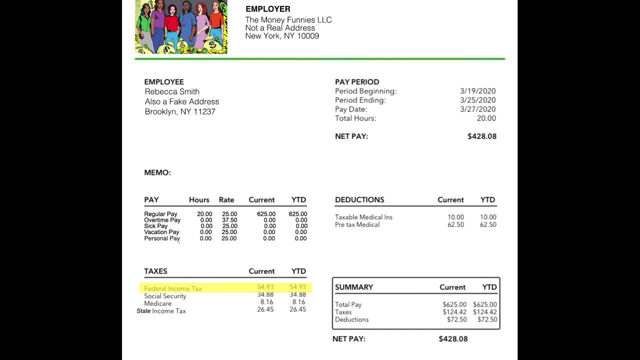 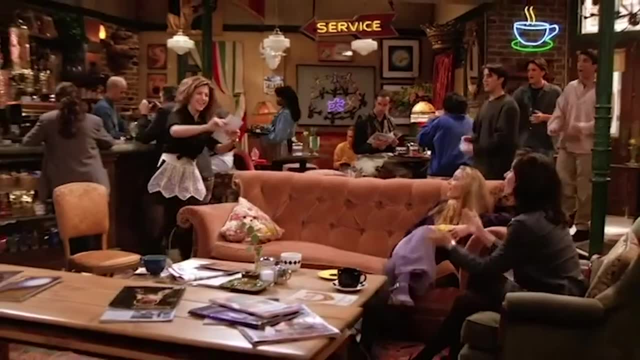 We spoke about that in detail previously, so I won't go into it again. Then we have FICA, Medicare and or Social Security taxes. This looks like my first paycheck. Look at the window. There's my name. Hi me. 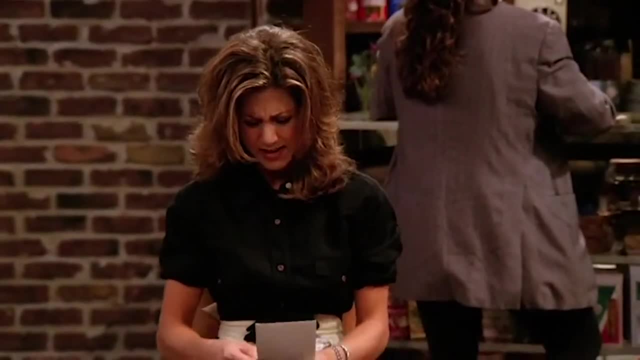 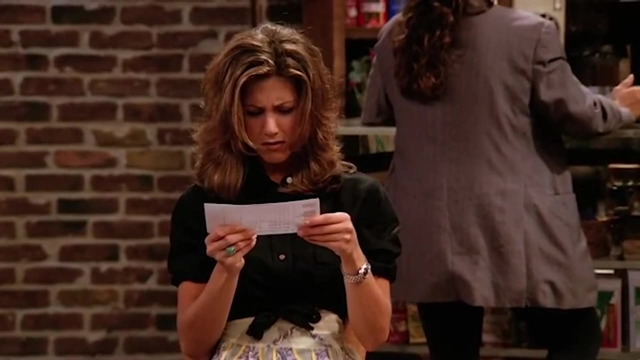 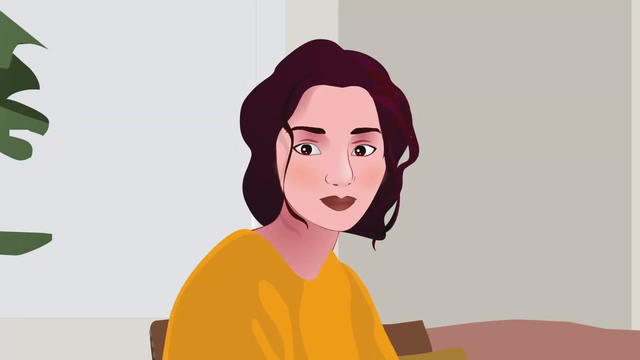 God, isn't this exciting. I earned this. I wiped tables, I wiped tables for it, I steamed milk for it and it was totally not worth it. Who's FICA? Why's he getting all my money? These taxes are charged to working people to pay for Medicare and Social Security. Those are federal programs that provide benefits for retirees, people with disabilities and children of deceased workers. They are sometimes known as payroll taxes. They are charged on all working income, regardless of how much money you make. They are not charged. They are not charged on passive income from investments like stocks or bonds. There are some exceptions, but they are rare. Okay, so they are a flat tax. It doesn't matter how much I make. Well, they are a percentage of what you make, but they do not follow the tax bracketing system we discussed. that applies to federal income taxes. 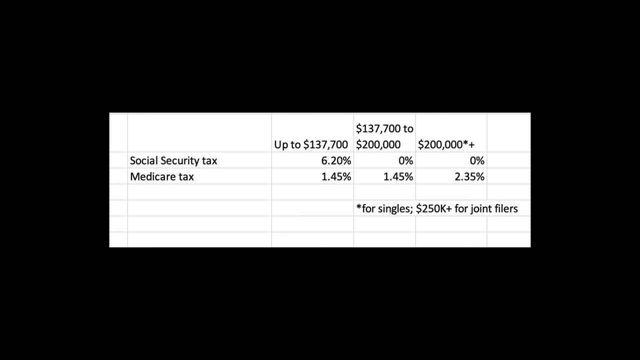 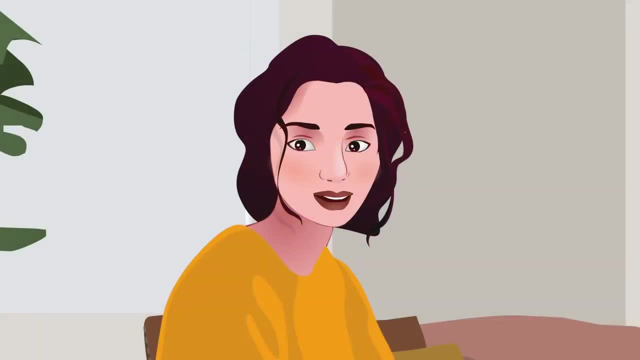 So nearly everybody pay a 7.65% tax to FICA. Got it? We all pay a 7.65% tax to pay for Social Security and Medicare. Lastly, we have the local income tax. Many states charge income taxes. 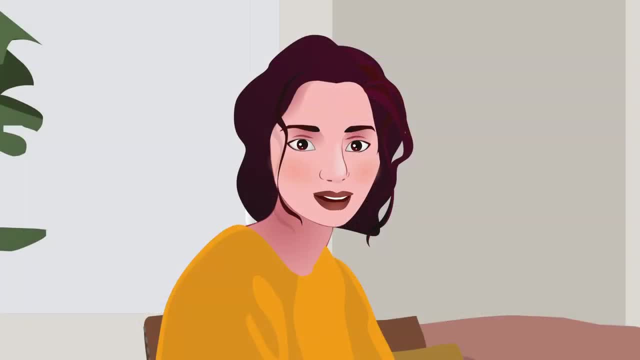 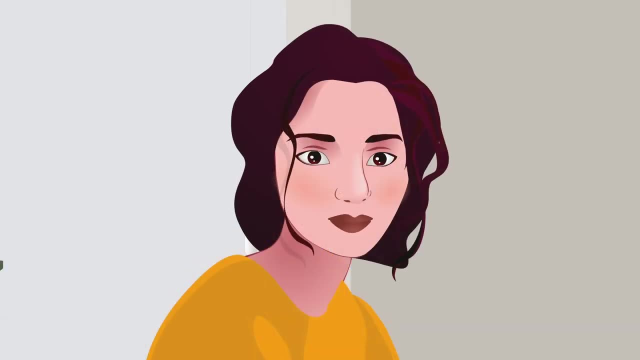 Most states charge income tax. This can either be the state where you work or the state where you live. You don't pay them to both states, But if one state charges income tax and the other doesn't, you'll owe the income tax to the state that charges it. Double taxation is not allowed. This is a bigger topic, so we should probably discuss it another week. So that's it. No, that's the federal and state taxes. Your local government, either where you work or where you live, may charge a municipal tax.